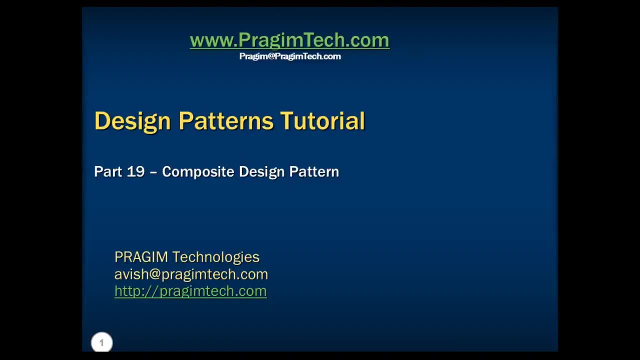 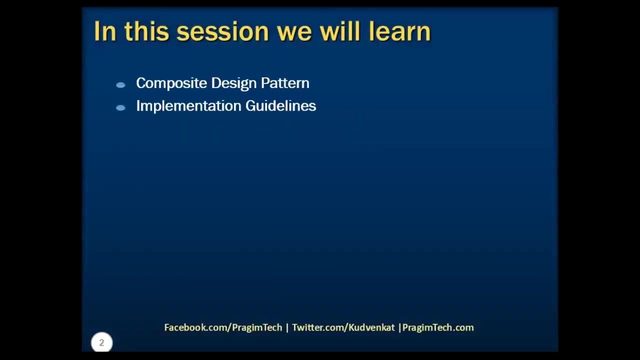 Hello everyone, welcome back. This is part 19 of the design patterns tutorial. In this session, we will discuss what is composite design pattern, implementation guidelines of composite design pattern, and we'll take a look at a simple example to implement this pattern. Please refer to the 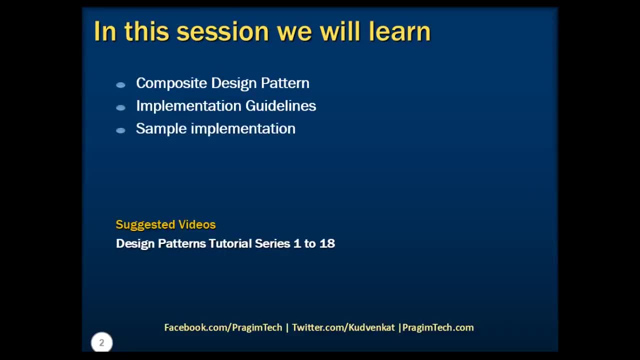 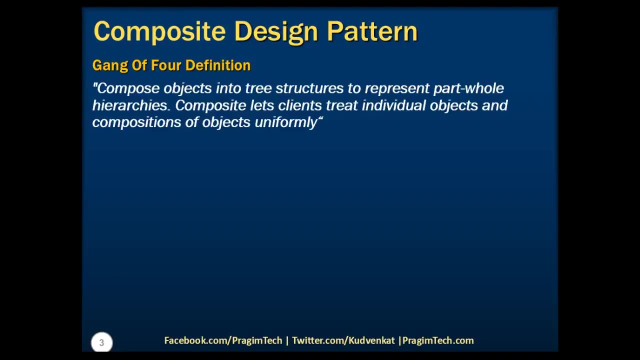 previous parts of the tutorial before proceeding. As per the Ganga 4 definition, composite pattern states that we need to compose objects into tree structures to represent part-whole hierarchies. Composite lets client treat individual objects and composition of the objects uniformly. Let's. 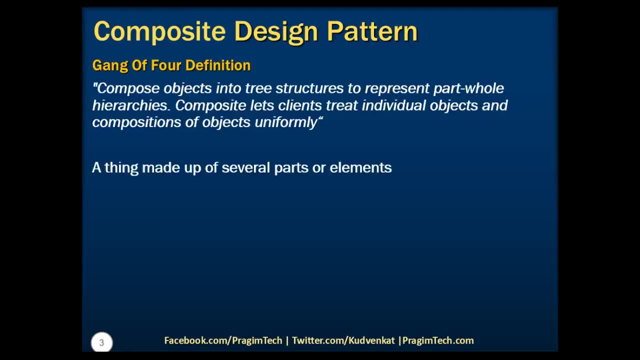 first understand what composition means. Composition means a thing made up of several parts or elements. In software engineering, the composite pattern is a partitioning design pattern. So we can say that the composite Composite pattern describes a group of objects that is treated the same way as a single instance. 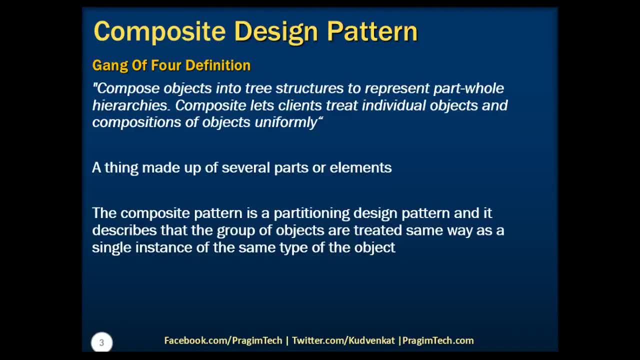 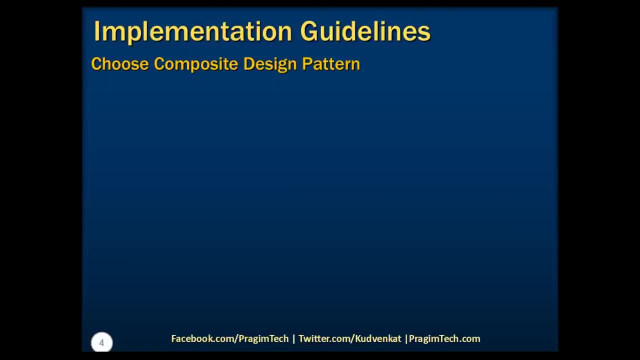 of the same type of the object. Let's now take a look at the implementation guidelines of composite design pattern. We need to choose composite design pattern when we want to represent part-whole hierarchies of objects, When we want clients to be able to ignore the differences between composition of objects. 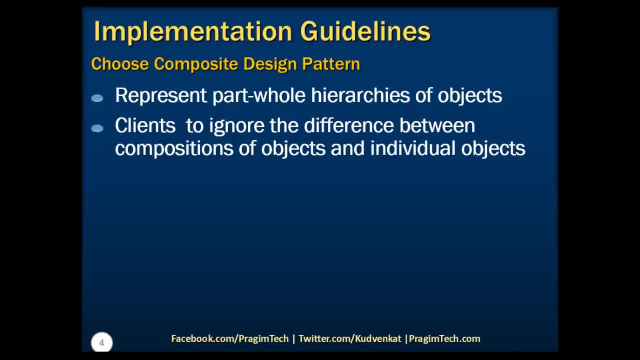 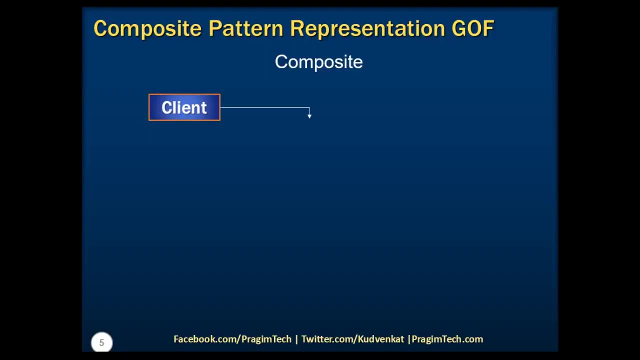 and individual objects, which means clients will treat all objects in the composition structure uniformly. Let's now take a look at the representation diagram of composition design pattern. as per the Ganga-4 definition, Clients use the component interface to interact with objects in the composite structure. 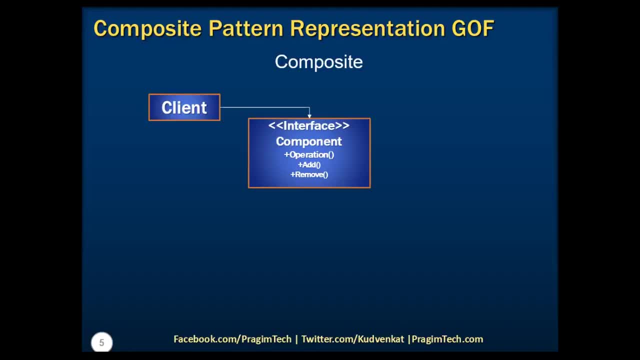 Component is the abstraction for all components, including composite ones. Component declares the interface for objects in the composition and the leaf represents leaf objects in the composition. leaf implements all the component methods. the composite represents a composite component. please note that composite components have children and they could be composite child's or leaves also composite. 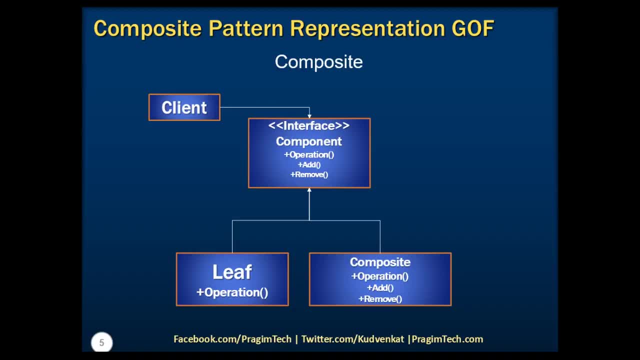 implements methods to manipulate children. composite also implements all component methods generally by delegating them to its children. if you take a closer look at this representation diagram, the composite pattern can violate the Liskov substitution principle, as we end up with a dummy implementation of add and remove methods at the leaf throwing runtime. 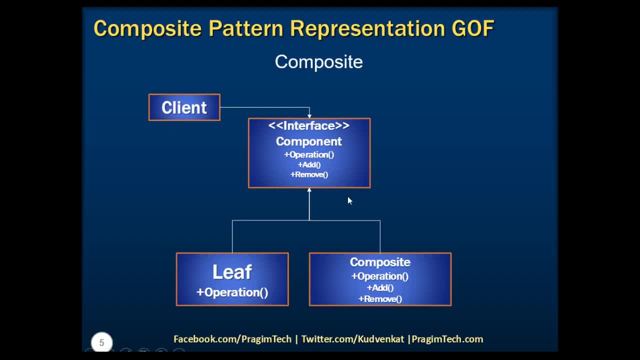 error as add and remove operations at the leaf doesn't make any sense or significance. however, at this point of time, Liskov substitution principle is out of scope of further discussions. hence we strongly recommend you to refer to the Liskov substitution principle session for more details. now, coming back to our current, 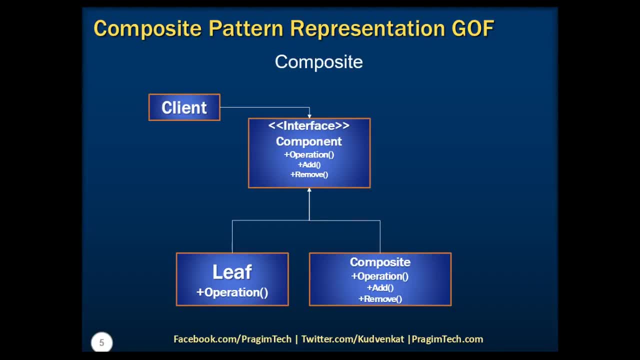 discussion, we should always keep in mind that a design pattern is a general, repeatable solution to a commonly occurring problem in a software design. of course, applying design pattern with the solid principles brings our best efficient code practices with problem solutions. however, our goal is to represent the part and whole. 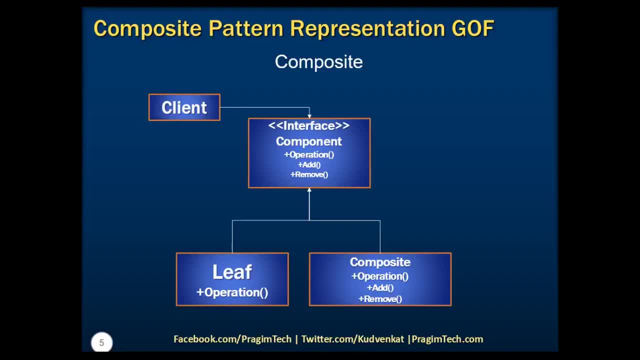 hierarchy of the objects in a same way. hence, we can change this representation slightly in a new form as shown on the screen. if you compare the previous and the current one, notice that we have changed the component methods to have the one which can be implemented by both leaf and composite nodes. additionally, we 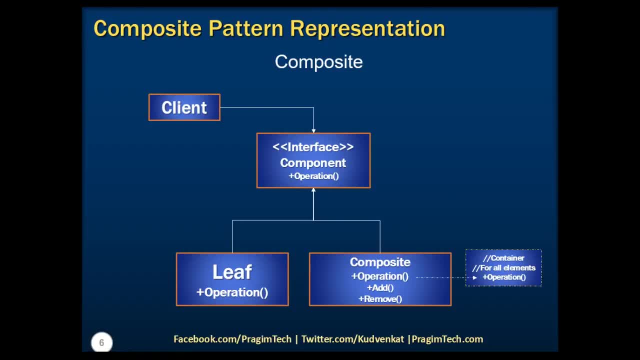 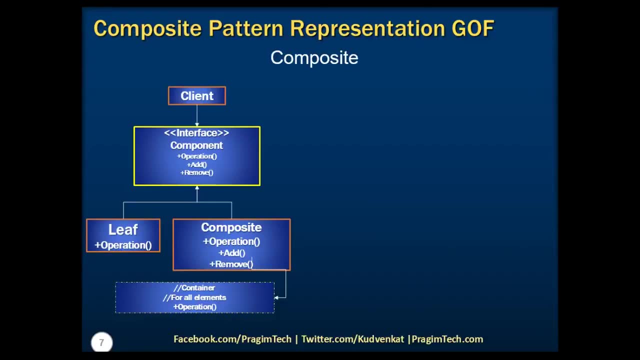 have add and remove methods at the composite level. Let's take a look at another representation diagram with a comparison. Notice that at the component level we have changed it a bit to adhere to the solid design principles. After all this, you might be wondering what is composite, what is leaf and what's all? 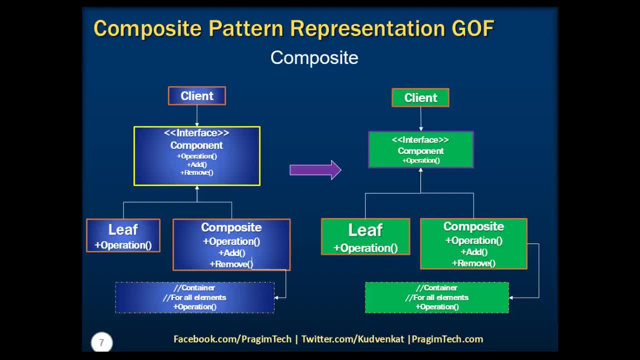 this design pattern about To answer that. we have many day-to-day example usage of this design pattern. Some of them are the computer representation, which consists of a system with a hierarchy, also an organization with an employee structure, which has employees as well as their managers. 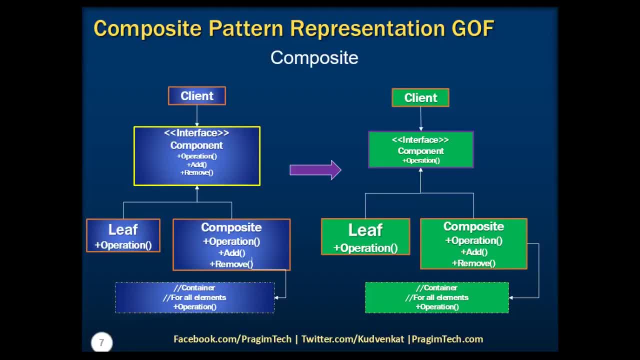 in different departments And, of course, in a day-to-day life of a person's family tree structure can be represented as composite design pattern. Let's now switch to Visual Studio and see how we can implement this with a simple example. To save some time, let's take a look at another example. 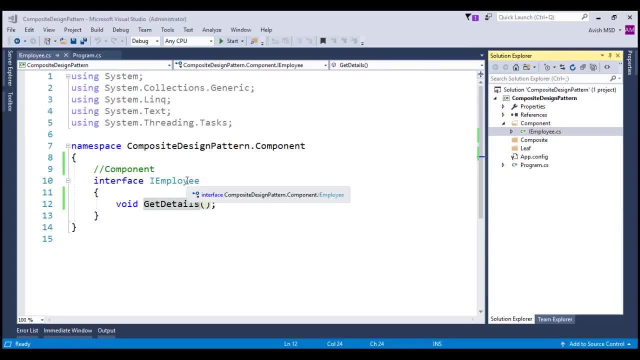 To save some time, I have already created a console application and created an interface called IEmployee, which has a single method implementation to retrieve the employee details. This interface is a component of this application and for representation purpose I have created a folder called component and moved this interface under this component folder. 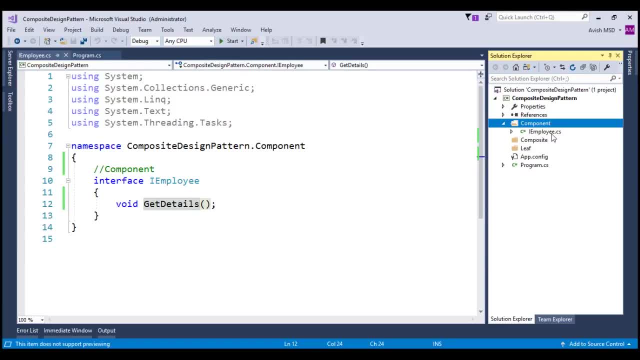 Again, I would like to reiterate that it's not mandatory to follow this folder structure, as we are just doing this. Now we need to create an employee that implements this interface, and please note that the employee will be the leaf of the organization. 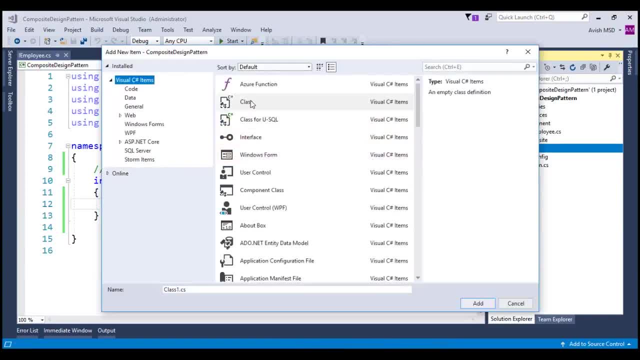 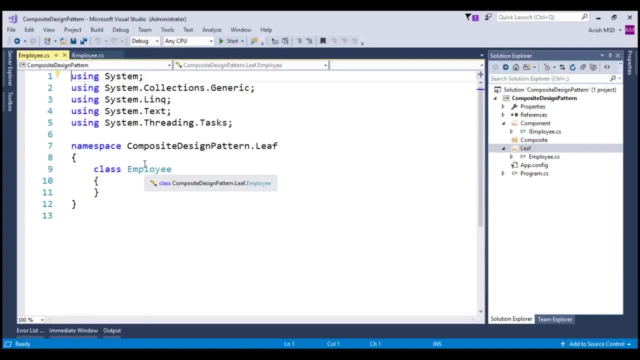 Let's right click on this leaf, add new item, choose class. let's name this class as employeecs and this will be our leaf class. So let's replace this code with the code which I have in my notepad to make the things faster. 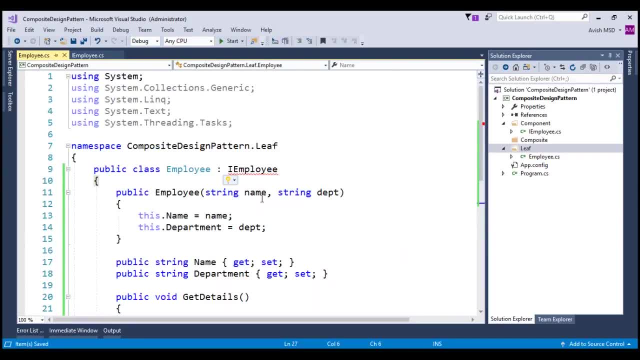 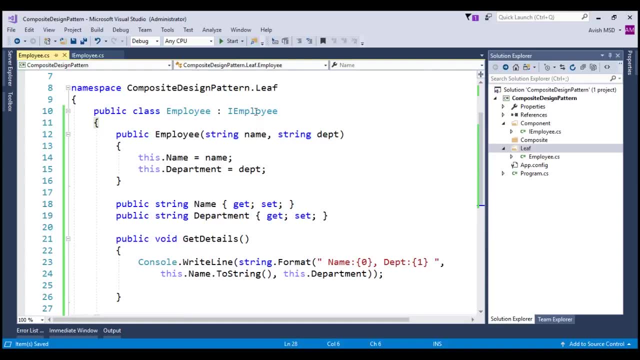 Now let's solve this issue by using interface implementation. Notice that we are inheriting the IEmployee, which is a component, and the employee, which is a leaf, and we are implementing the getDetails method. We are just printing the name and department of this employee in the getDetails method. 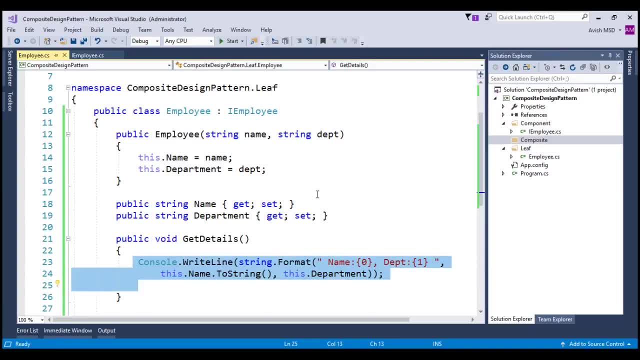 to the console program. Let's say we need to classify the employees in an organization, Then we would want to get all addEd fuerte functionality in this right. Not that we need to outright separate the information because if we don't want that blow. 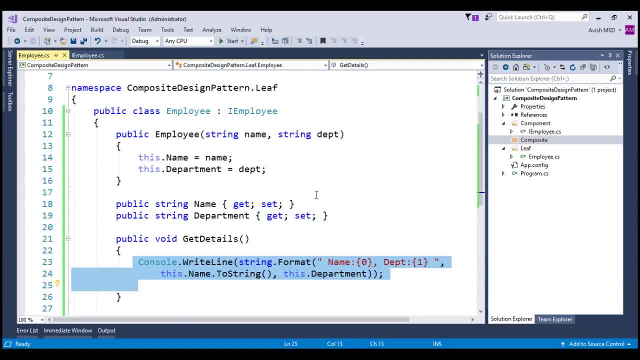 out. you just need that purposes item AND we would want to play with how essentially the name the person belongs on the class. To answer that, we just need to create manager who also manages the subordinates. So let's to pistol fire the finalium andschedule property of this component to the new one. 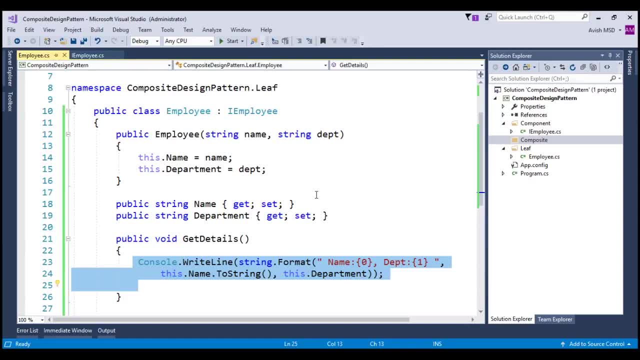 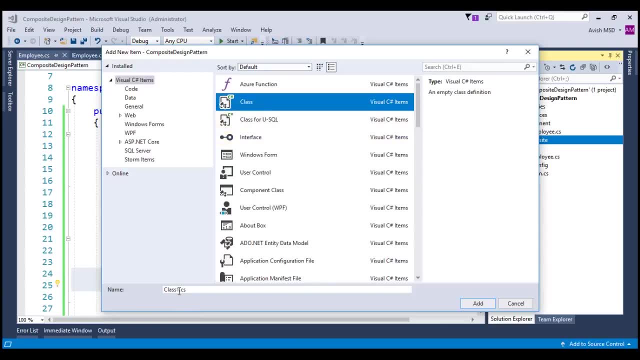 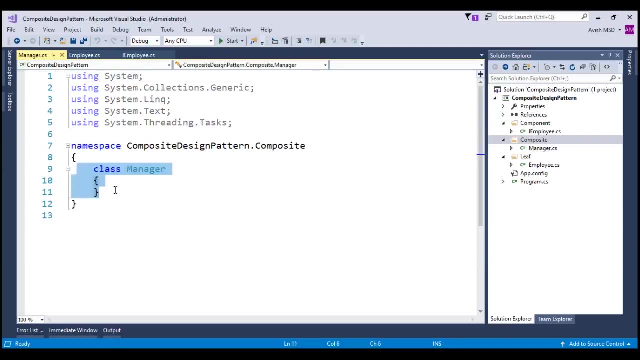 as a reference here. That's because I als this measure of the group being theGetDetail property, which I call component, and this chain class is the one that, if we want, we just win three time returns. a new item manager. to make the things faster, let me copy the code for this manager. 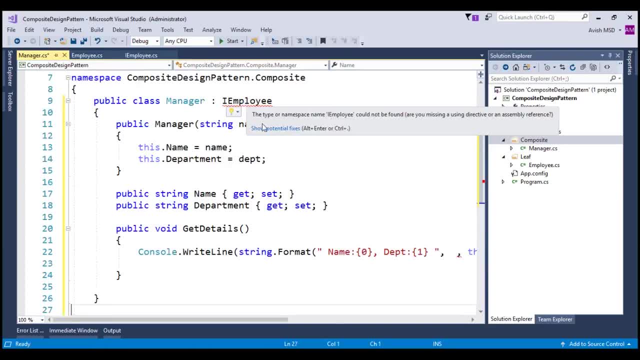 implementation. let's just all this missing references. now, as you know, that manager represents a composite component, which means manager has children which are called as subordinates, and that subordinates are the collection of employees who are reporting to him. so let's create the representation by adding list collection of employees and call them as. 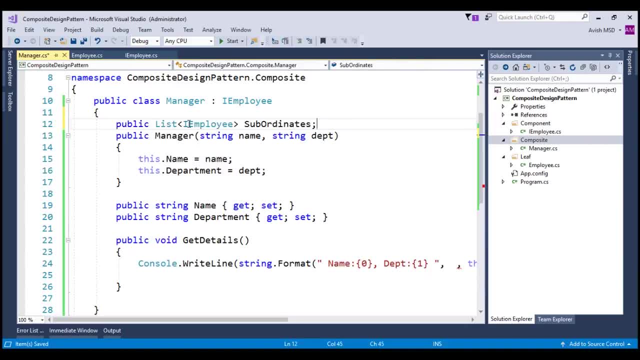 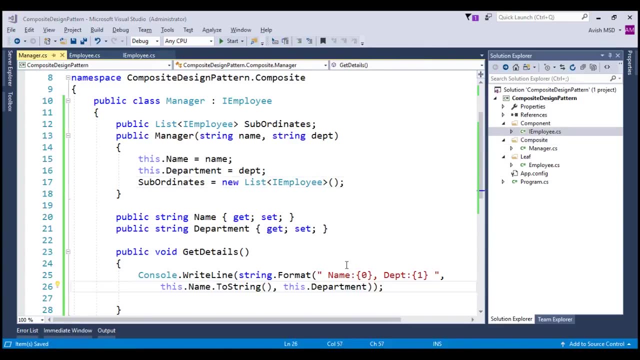 subordinates. let's quickly do that. also, let's initialize these subordinates in this constructor of manager, as discussed in the beginning of this session. we do not need to add subordinates to the list of employees, so let's just add subordinates to the list of employees. so let's just add subordinates to the list of employees. so we do need to implement all component. 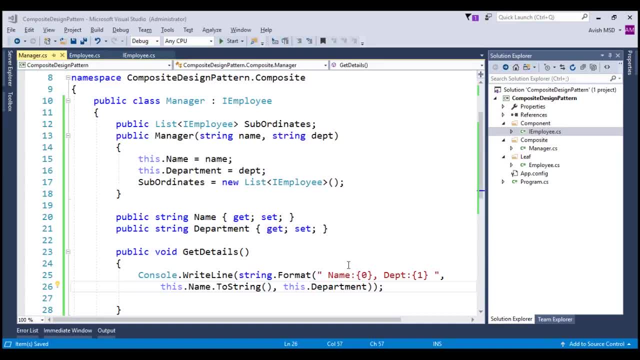 methods, and we achieve that by delegating them to its children. now, if you notice that in the get details method, we are just printing the manager details only, however, to retrieve the details of subordinates, we need to traverse through the child employees and get their details. so let's do that over. 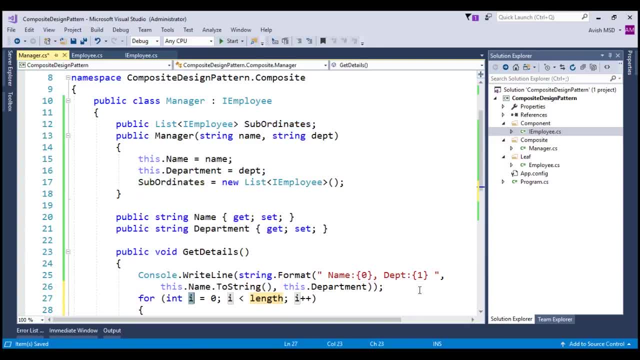 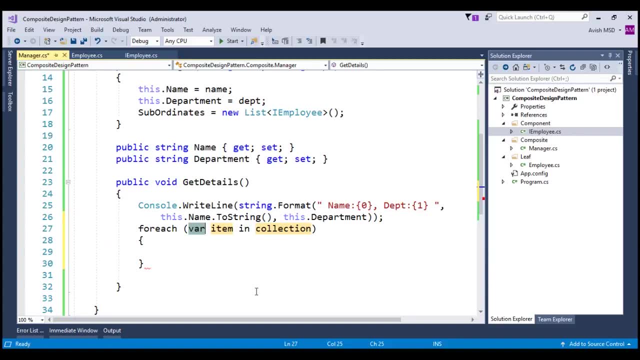 here for each. we can take for loop or for each loop. for our convenience let me take for each loop. or here see where employee in subordinate collections let's just print employee dot, get details. for each of these managers supernets, we are going to invoke the getDetails method, which is the leave method of employee, and notice that. 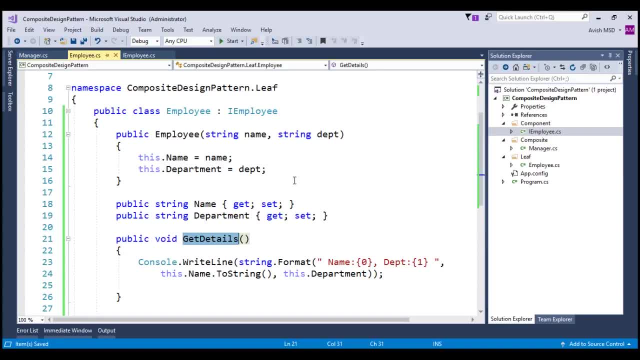 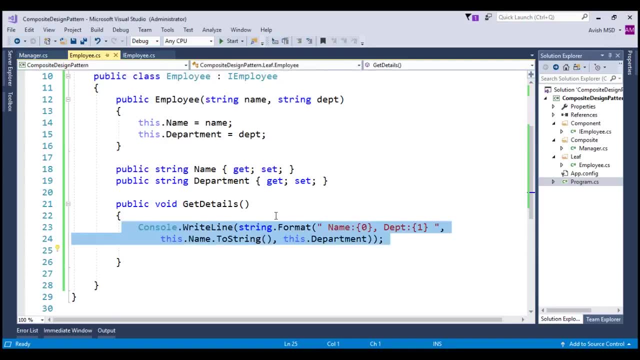 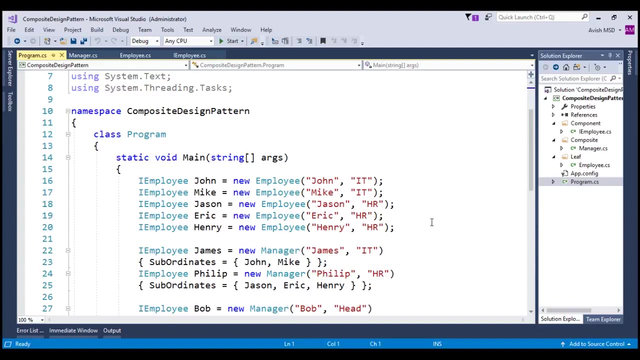 whenever it invokes the get details of the employee subordinates, it's going to print the employee details. now that we have created the component composite manager and leaf employee, let's use these in the client method, which is our console program. let's switch to the console program to make the things faster. I have already added few. 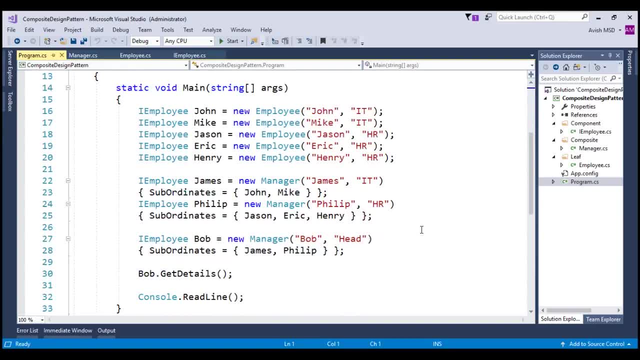 employees in the console program, notice that we have five employees who are John, Mike, Jason, Eric and Henry and they belong to ITN HR departments. also, we have created two managers, James and Philip, who belongs to ITN HR department and they manage ITN HR departments. we have also added their subordinates. 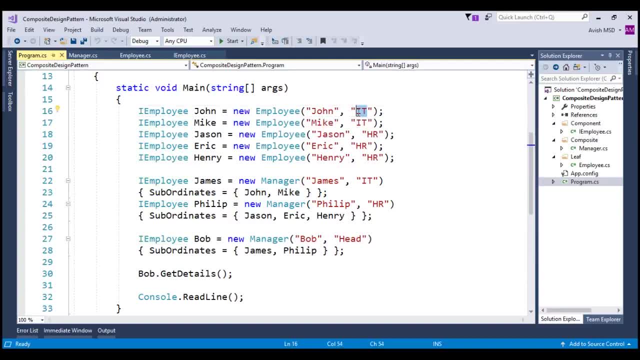 according to these employees who are in ITN HR department, we have also created both subordinates as well: Bob, who is the manager of this institution, or we can say that the Bob is the head of the institution, who manages both James and Philip, who belongs to IT and HR department, and they are the managers of. 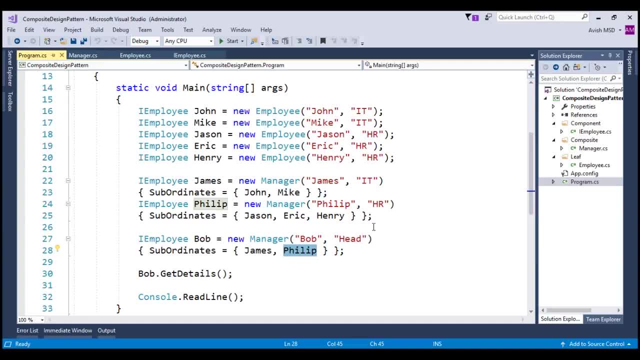 IT and HR department. Now, if the end client need to get the details of Bob, we retrieve the details of Bob, as well as his managers and his subordinates, because Bob is acting as a composite manager here which traverses to the other composites, as well as the leaves. 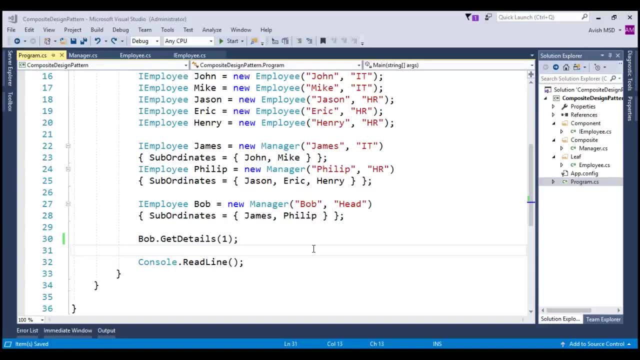 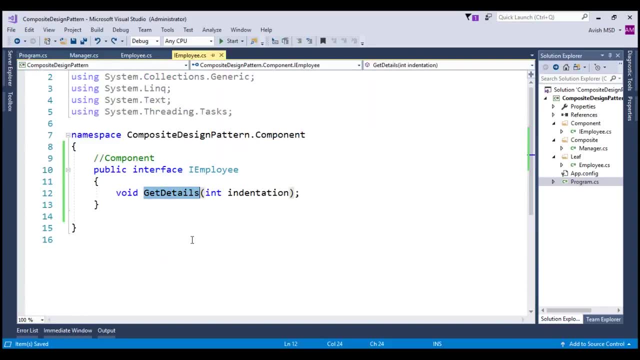 To make the output represent as a hierarchical structure, I have modified the methods to print a visual indentation for managers and employees. Notice that we have added a parameter called indentation, which is also a visual indentation. Now, if the end client needs to get the details of type integer also, we have changed the implementation of get details to add this. 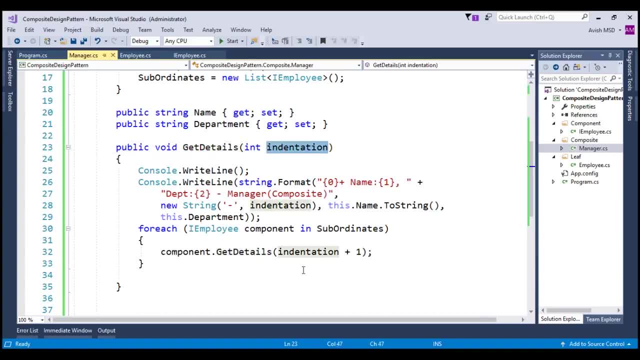 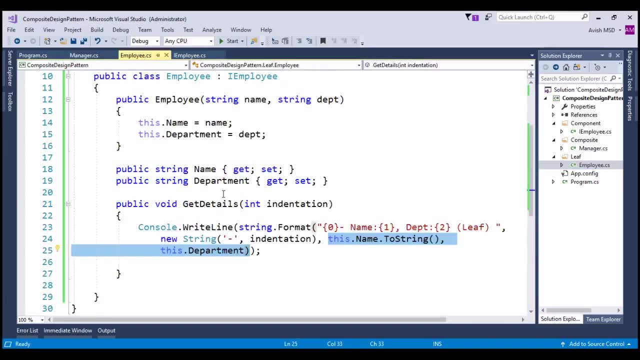 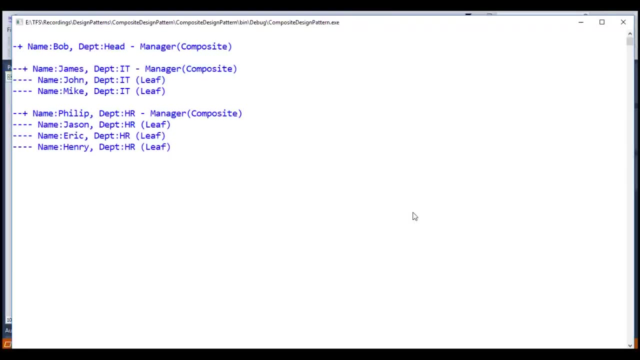 indentation before printing the name and department for the visual representation. I have done these changes both in the get details of manager as well as employee. to make the things faster, Let's run this application now. Notice that we have the complete composition details of the Bob. 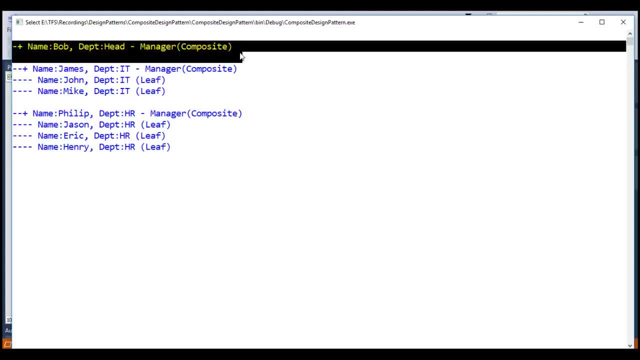 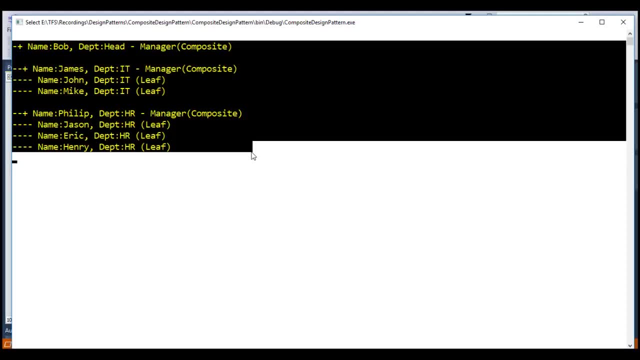 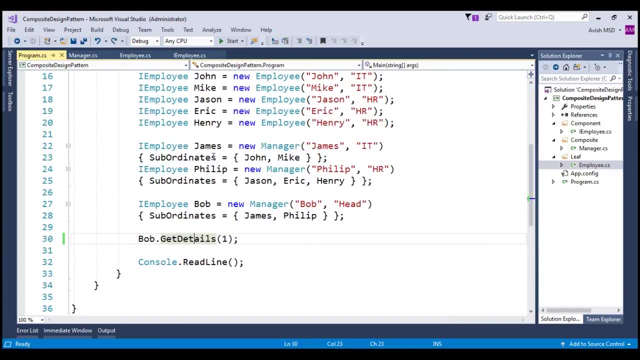 Who is the head of the department and his subordinates, who are James and Philip, along with their subordinates, which are the leaf employees. Now let's switch back to this application and do a little change over here. instead of retrieving Bob's get details, let's retrieve James dot get details, and.